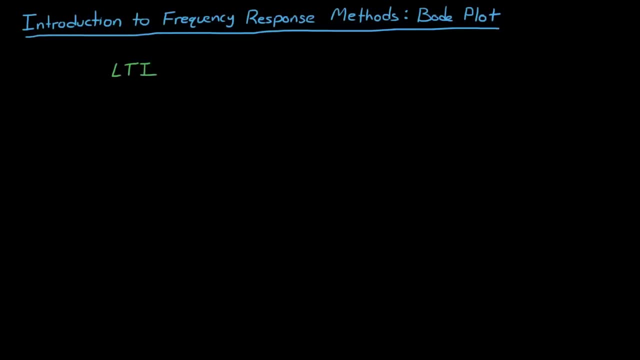 I want to start by explaining another benefit of an LTI system. If you design a linear time invariant system, then there's only a limited number of mathematical operations that you can use When building an LTI system. you can only use one is multiplication by a constant. the second is differentiation of the input signal. the third is integration of the input signal. 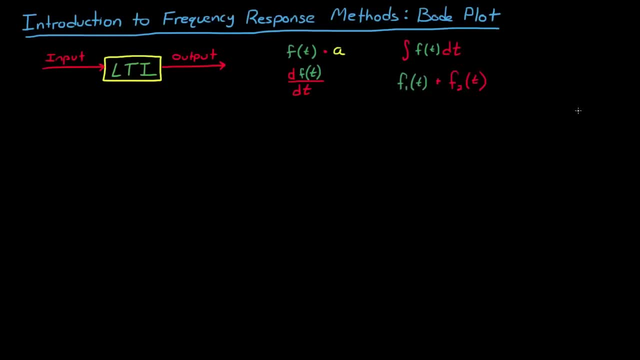 and the fourth is multiplication of the input signal. The fourth is adding two inputs together. You can always do division by multiplying by the reciprocal, and you can also subtract by adding a negative number. You might be wondering why it's important for me to start this lecture this way and why bring up the fact that a linear system can only consist of these six operations. 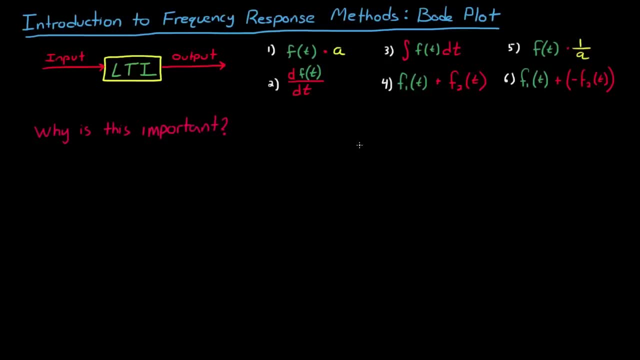 The answer is that when you subject a sinusoid to these operations, it doesn't change shape, And part of not changing shape means that it also won't change. A sinusoid will always change frequency. A sine wave input will always generate a sine wave output of the same frequency. 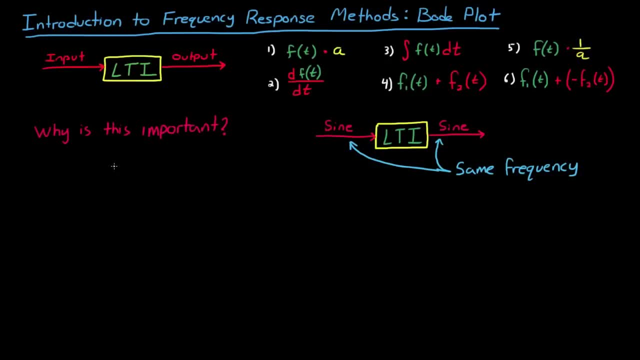 In fact, the only two differences possible between an input sine wave and the output sine wave that's generated is the amplitude, which is the height of the sine wave, and the phase that is shifting the sine wave in time. In fact, the sine wave is the only repeating waveform that doesn't change shape in a linear system. 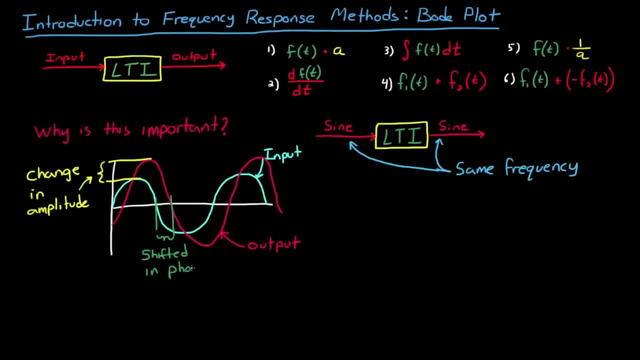 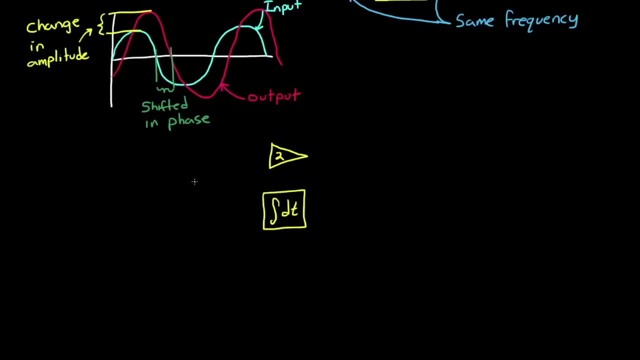 You can see here graphically what it means to change in amplitude and also to shift in phase. Let me give you a quick example so you can see what I mean. If we take an input sine wave and subject it to these two separate paths, the upper path is just multiplying it by a constant 2, and the lower path is integrating it and then summing them together produces the output. 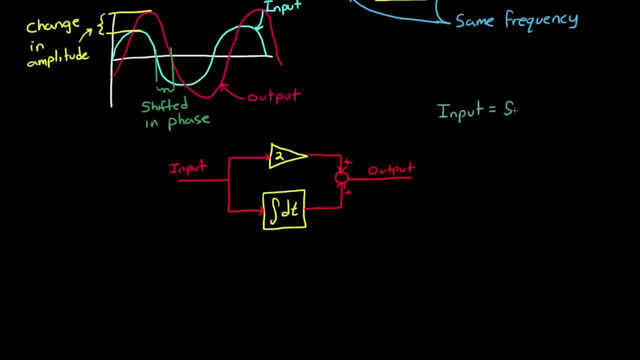 If we make the input a pure sine wave of frequency- one-half radians per second, then we can just calculate mathematically what the output would be. I'd like to make a quick note about frequency. I'm going to refer to frequency in units of radians per second, but this is proportional to hertz. 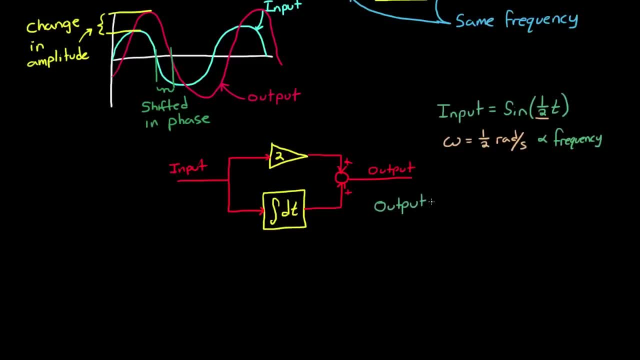 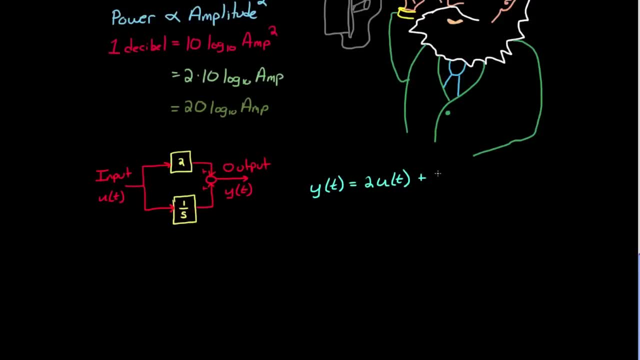 We can simplify this further by just taking the integral of the input with respect to time. Now writing the transfer function for a system like this can be done. The output y of t is equal to 2 times the input u of t plus u of t divided by s. 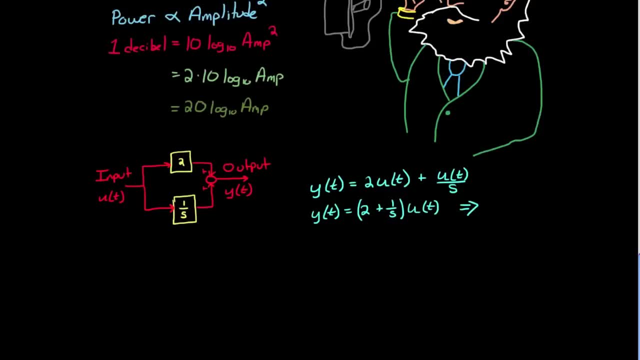 A few algebraic steps here and you can solve for y of t over u of t, which is the transfer function, which is equal to 2s plus 1 divided by s. Recall that the Laplace transform s is a complex variable, sigma plus j, omega. 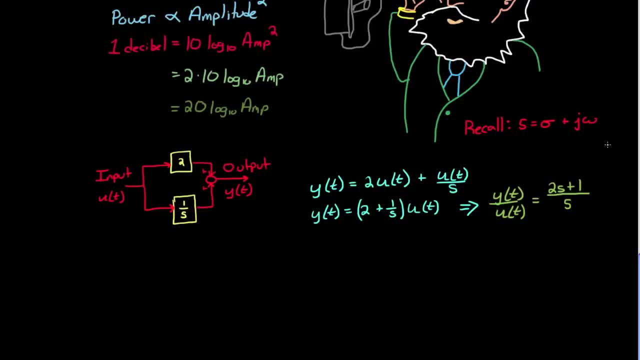 However, when we're talking about frequency response of a system. However, when we're talking about frequency response of a system, we are talking about the steady state response, That is, once all the transients have died out, or in other words, when the exponential term sigma is zero. 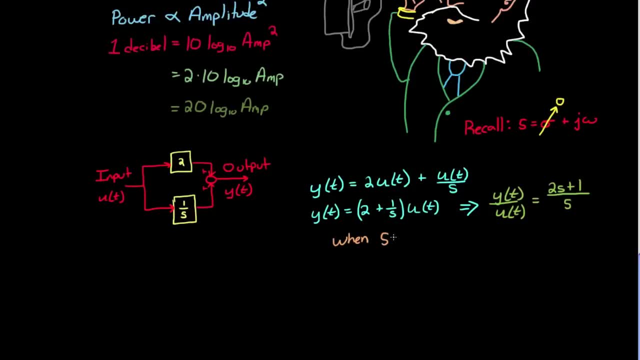 So for steady state behavior, s just becomes j omega. Steady state phase and gain can be calculated directly from a transfer function by setting s to j omega. That makes the transfer function become 2 plus 1 over omega j, where 2 is the real component and 1 over omega is the imaginary component. 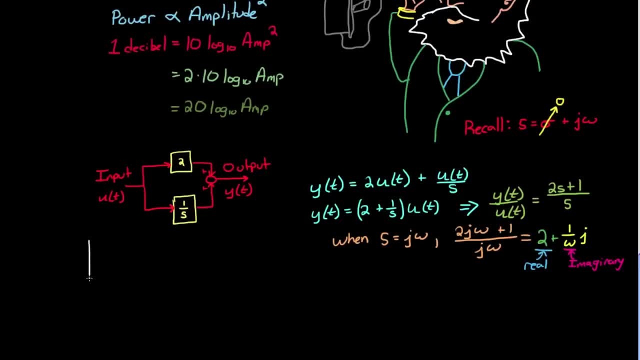 If we then plotted these real and imaginary components on a real and imaginary axis, then we can calculate gain and phase geometrically from this plot. So here our real component is 2, and for omega of 1- half from our example above 1 over omega would also be well, it's negative 2.. 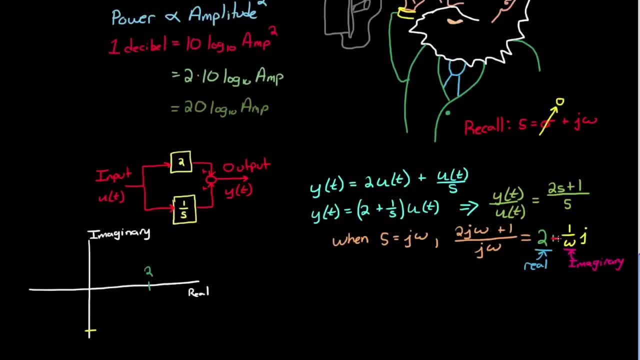 I'm sorry I made a mistake here. This 2 plus 1 over omega should actually be a minus, because j times j is negative 1.. So it's negative 2 on the imaginary axis for omega of 0.5.. And if we draw a line from the origin of the axis to that point, 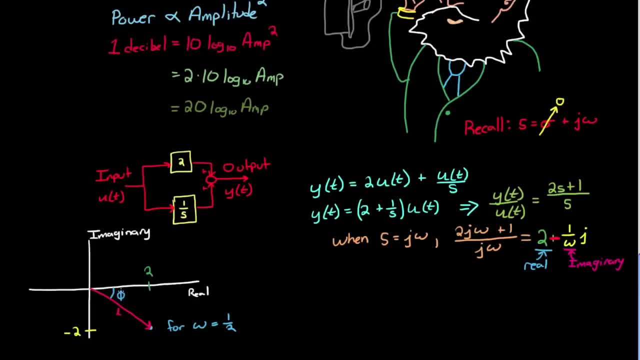 then the length of the line is the gain of the system, And the length can be calculated by just taking the square root of the real component squared plus the imaginary component squared. This is just the Pythagorean theorem, And the phase is the angle between that line and the positive real line. 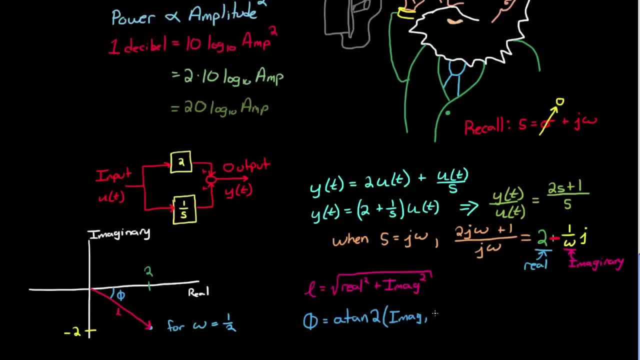 And you can solve for this using the arctangent. I'm using arctangent 2 in this case only because it keeps track of the sign of the inputs, and so you don't have to worry about whether a is positive or negative, like we did up above. 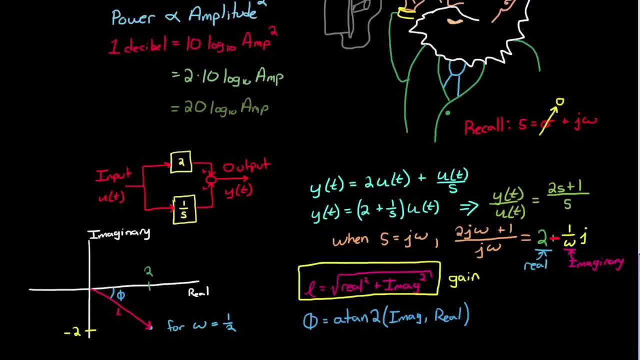 So again, the length of this line is the gain and the angle off the positive real line is the phase. So you can see in this example that the real component doesn't change with frequency, only the imaginary component. And if we sweep through this, 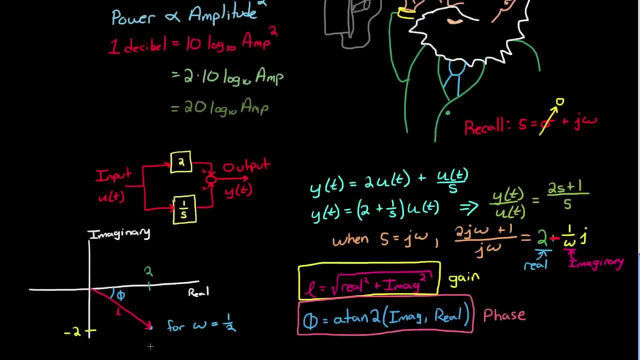 through frequencies from near 0 all the way up to near infinity, you can get a visual understanding of what the gain and the phase are doing for this particular system. At omega of near 0, the imaginary component is almost infinite, And at an omega of near infinity, the imaginary component is near 0. 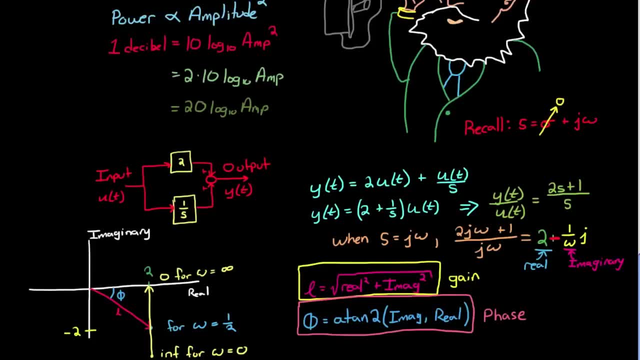 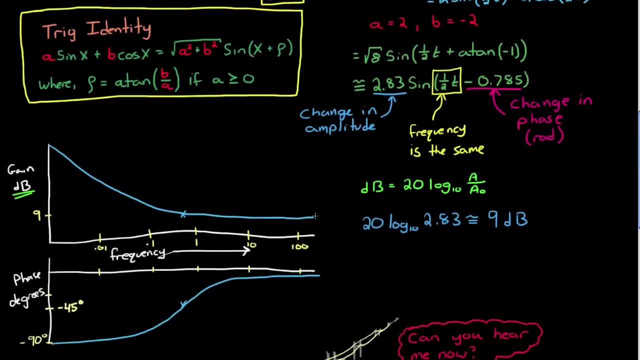 If we go back up to our plot, you can see. that's exactly what the gain is doing. The limit as frequency approaches infinity goes to 6 dB, which is a gain of 2.. And off to the left as frequency approaches 0,.